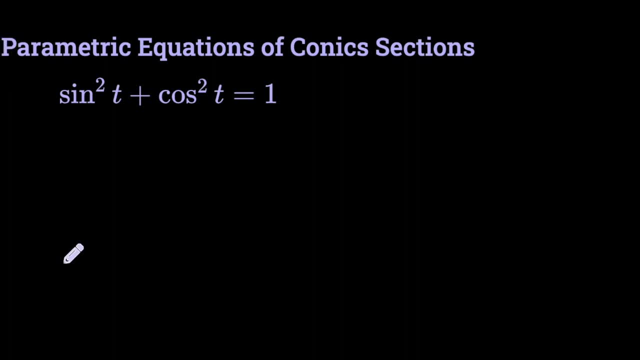 to yield the same conic section. So, for example, if I say: let x equal sine of t and y equal cosine of t, we will see that if we plug this in we would get x squared plus y squared equals one which we know as our friend, the unit circle. So in this case, if we let x, 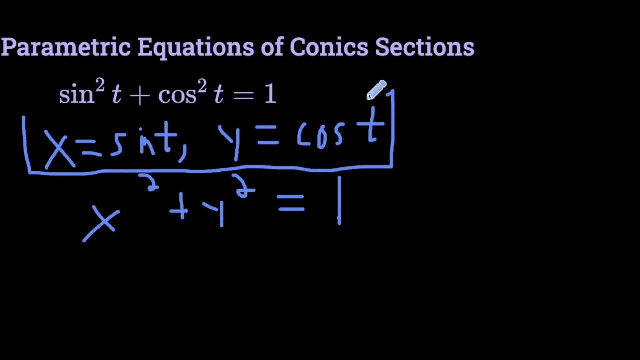 equal sine of t and y equal cosine of t be our parametric representations. remember from before, parametric representations mean we define x and y independently in terms of t. So in this case we would have a definition of the unit circle. Now, if we think about 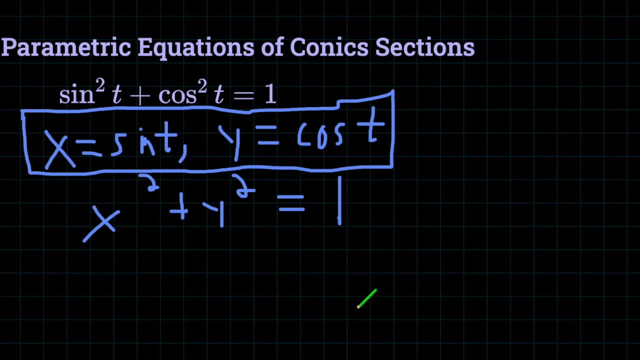 what that would look like. let's draw ourselves a little picture And let's think about different important values here. So when t is equal to zero, it would be sine of zero, which is zero, and cosine of zero, which is one. So the point would be zero comma one, which is up here. And then when I plug, 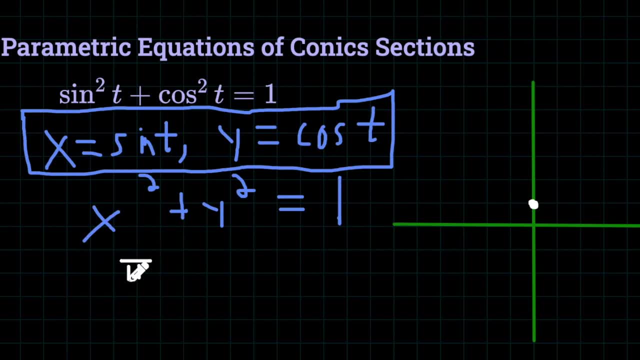 in our next important point: pi over two. sine of pi over two is one. cosine of pi over two is zero. and so we're down here. So we're graphing the unit circle, starting from up here and moving in the clockwork. 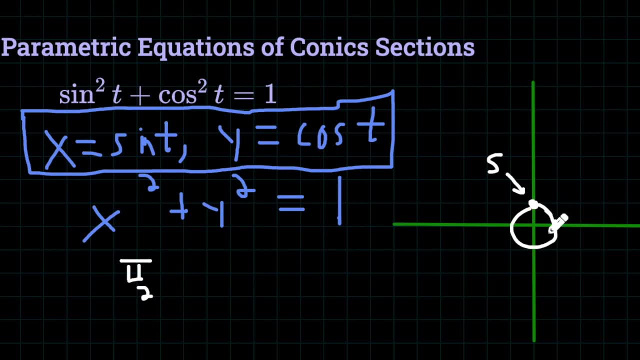 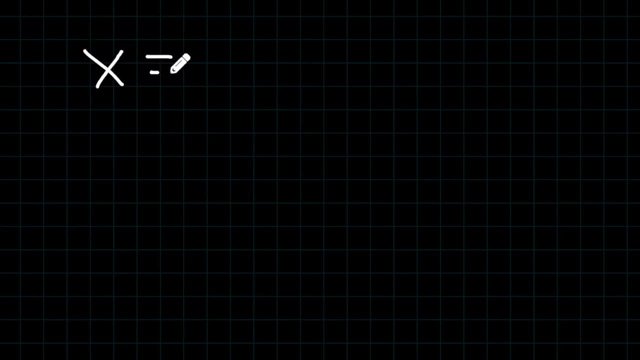 And then we can see that we have x equal sine of t and y equal sine of t. Now if I instead done a parametric representation where I said: let x equal cosine of t and y equal sine of t, I again still have the relationship that x squared plus y squared is equal to. 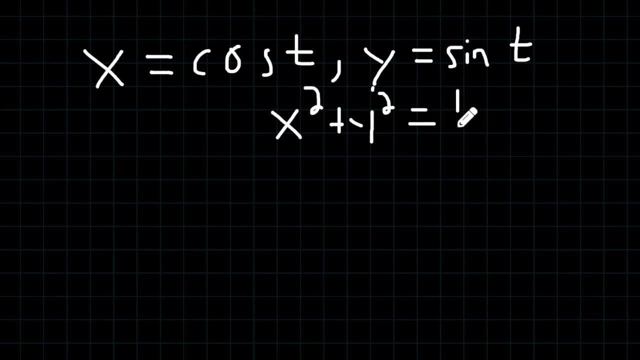 cosine squared plus sine squared, still equal to one. However, if I go and graph it this time, if I plug in the value t equals zero, t equals zero would be cosine of zero, which is one, sine of zero, which is zero. I'd be starting. 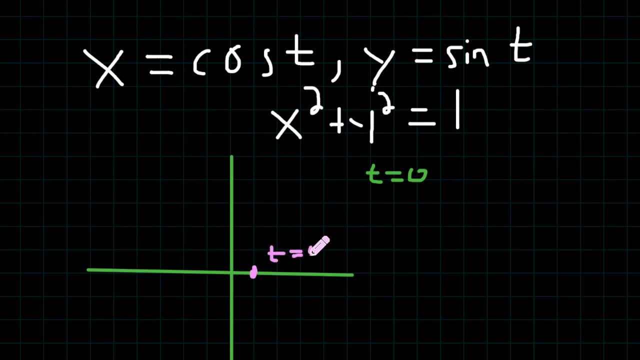 here when t equals zero. So then let's see where I end up as I move along. If t is pi over two, we know that the cosine of pi over two is zero, and the sine of pi over two is zero, of pi over 2 is 1, so we actually go here. So in this case, our unit circle starts on the x-axis. 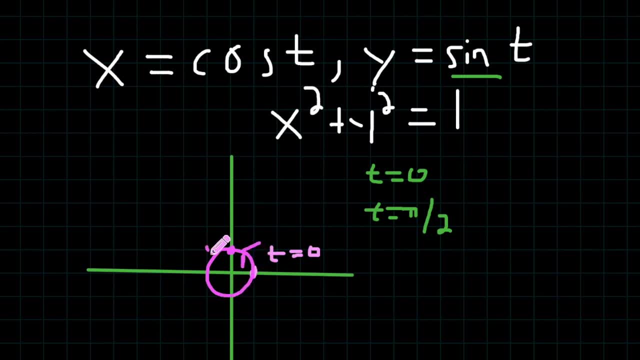 and moves in the counterclockwise, the sort of trig direction that we're more used to. So, depending on how we make our parametrics, how we define our x and our y, we'll get the same shape right. We still get the unit circle in both situations. However, 1 starts on the x-axis. 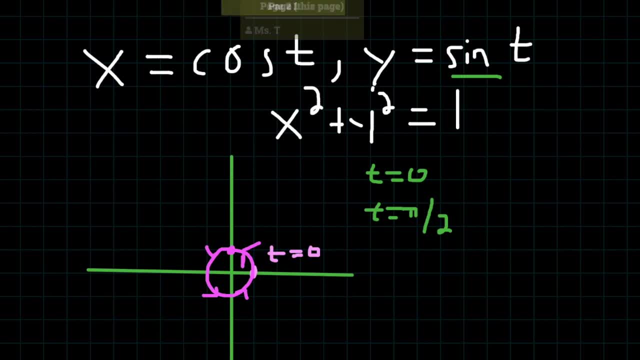 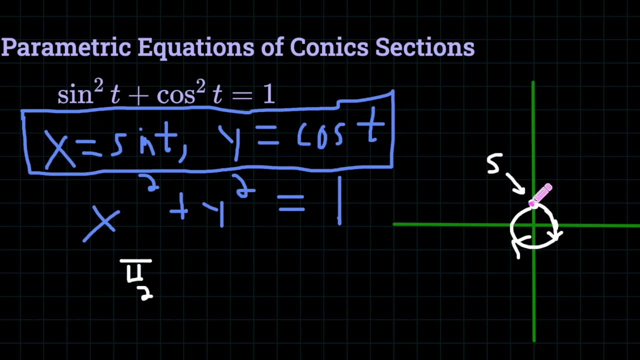 and goes counterclockwise, shown here. The other one started on the positive y-axis and moved clockwise. Could you think of any more? Are there any other ways to define x and y, such that x squared plus y squared still gives me 1?? There are, and I'll let you think about. 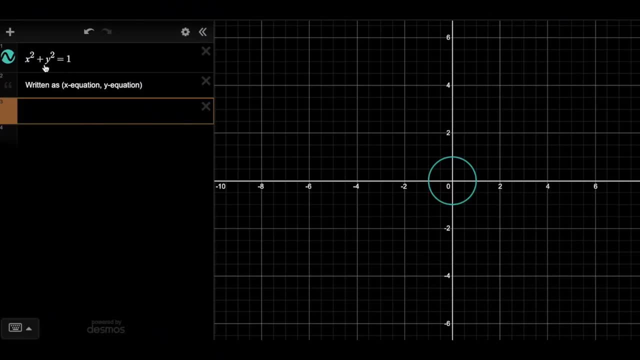 those for a moment. How to graph parametrics in Desmos. we can see we've written the equation for the unit circle up here, So I'm going to go with the more traditional, that x is defined to be cosine of t and y is defined to be sine of t. parametric version of. 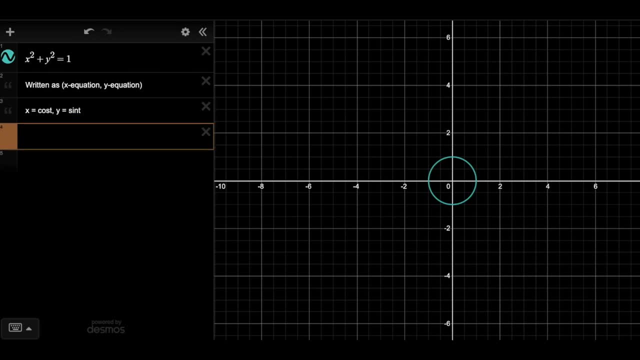 the unit circle. So the way we graph a parametric equation in Desmos is we write a set of parentheses, think an ordered pair, and we write the x equation first comma, the y equation second. So cosine of t, sine of t. And what you'll notice once I change the color to something slightly different, 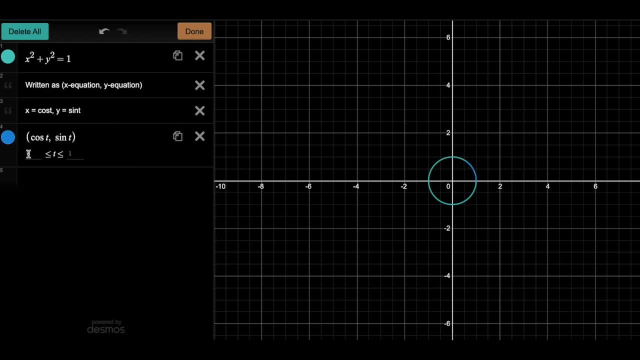 it's graphing this dark blue section Over here because it's only using the values from 0 to 1, right to get the whole unit circle we have to go. well, pi over 2 would just get me a quarter of the way there If I go by pi. 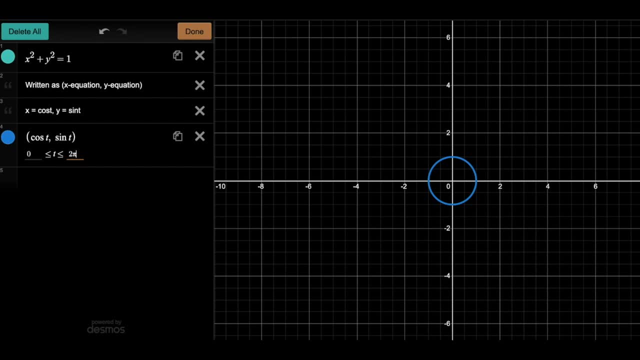 it's half the way To get the whole unit circle, I need to go a whole 2 pi. Another way that I like to represent this so I can actually see the direction is: I'm going to just use an unknown variable, So I'll call it a So. 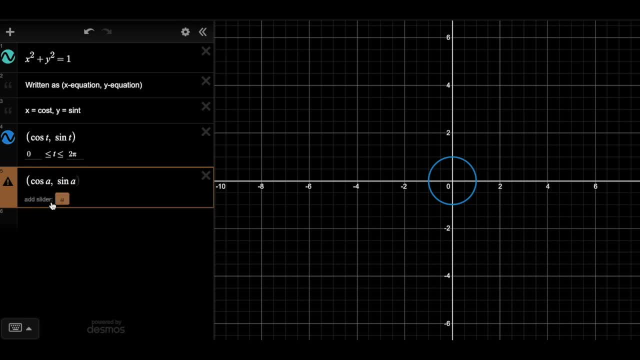 cosine of a and sine of a And we can add this thing called a slider. And so if I use the slider from 0 to 2 pi and I start it at 0, and then I hit play, I can actually watch it go around the. 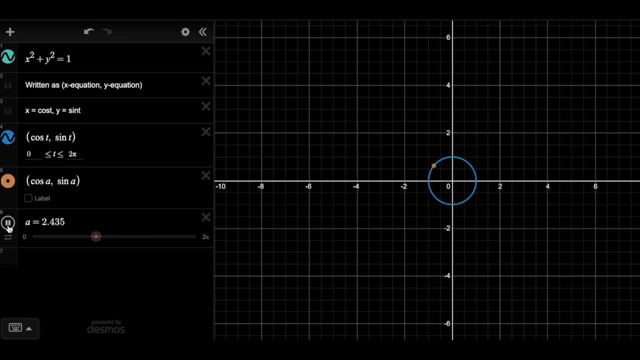 unit circle from 0 to 2 pi, And now it's going backwards. I can send it always to go in the same direction, So you can watch that as t increases. in this case it's just known as a. it's going. 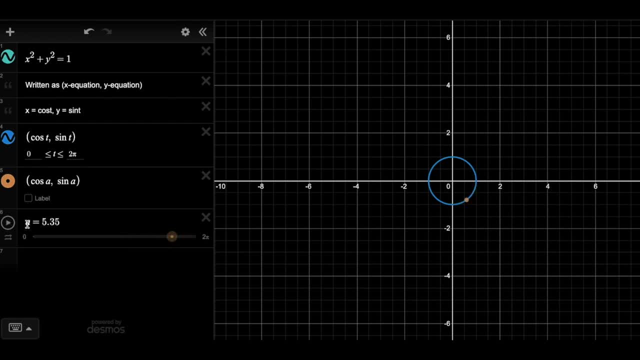 around the unit circle in the counterclockwise direction. We can also see that when t equals 0,, we're on the positive x-axis at the point 1, 0.. If we were to use an alternative representation of the unit circle, sine being the x, cosine being the y, now when we watch it travel around, 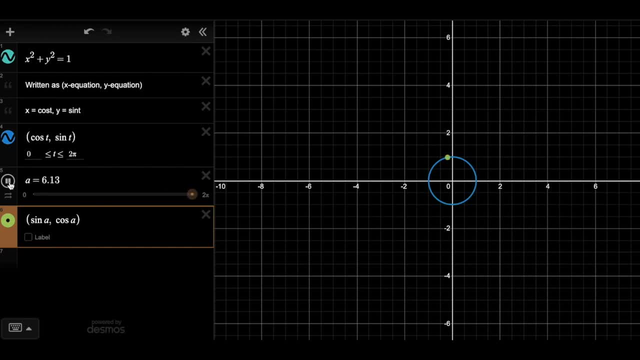 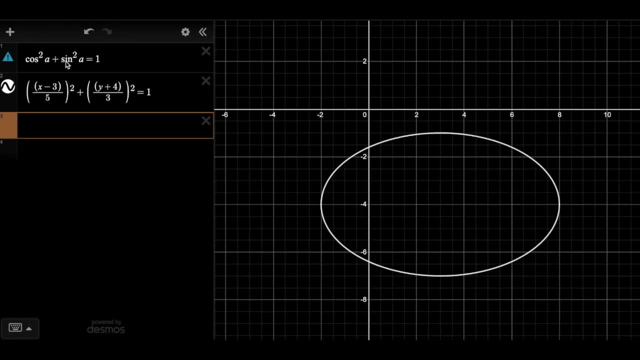 the unit circle. we see it starts at 0, 1.. And travels clockwise. How we would write parametric equations for an ellipse. So again, always remember: cosine squared plus sine squared is equal to 1.. So here's the equation of an. 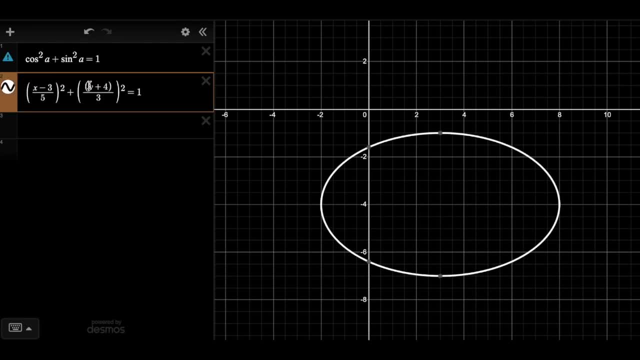 ellipse that I have over here And we're getting pretty familiar with the ellipse so we can recognize that the center is going to be at the point 3, negative 4, the hk value. We have an, a value of 5. a is with the x-coordinate because it's the center of the ellipse, And then we have 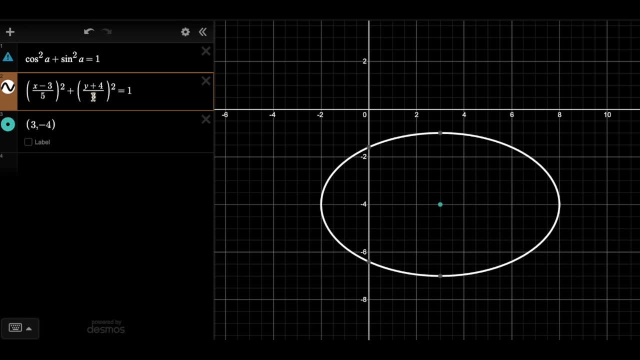 the largest. so this is a wide ellipse, and our b value being 3, and thus our c value would be 4.. But I want you to compare these two equations: They're both equal to 1.. So we can make a. 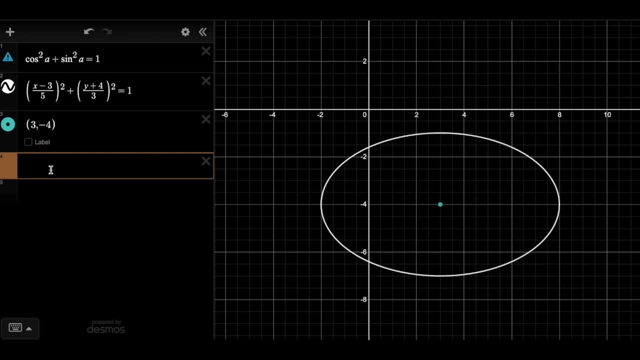 substitution. that would lead us to a similar situation to how we use the unit circle. So in this case I'm going to say let cosine of t. this could be any variable, a, t, whatever you'd like, I'll use t. Cosine of t is going to be defined as everything inside. 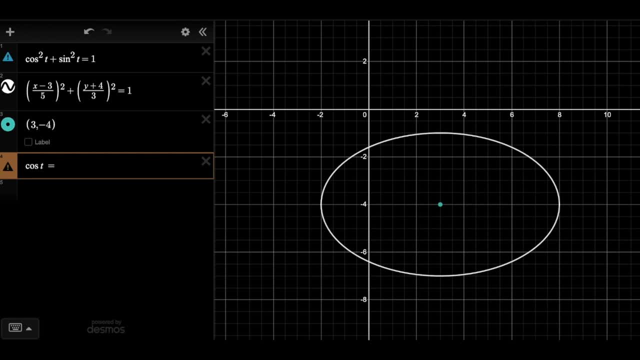 my first parentheses, So x minus 3, all over 5.. And in a similar way, sine of t is going to be equal to y plus 4 over 3.. And then if I solve for x and y, we see that x is equal to 5 cosine t plus 3.. 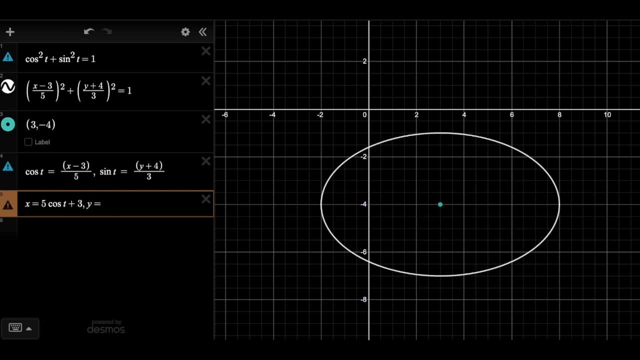 And y is equal to 3 sine t minus 4.. So now if I go into Desmos and I graph my parametric, which, remember, we just used parentheses, So that's the x equation, the y equation And you see, we've got this little lime green section over here. If I go 0 to pi, we get half the ellipse. 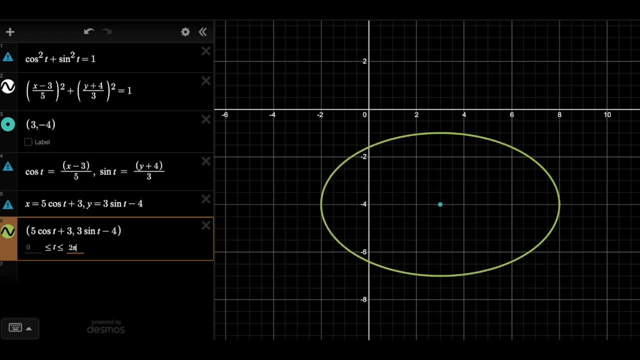 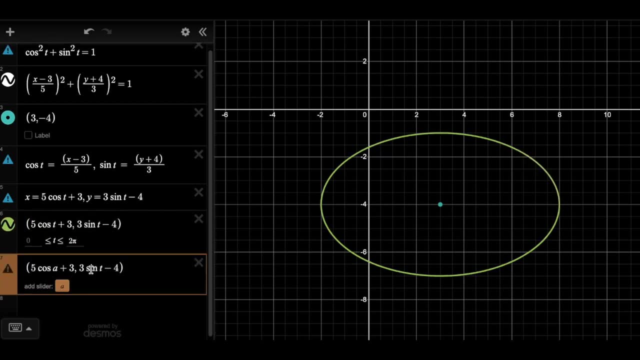 almost called it a circle. It's definitely an ellipse And if I go the whole 0 to 2 pi, you can see the entire ellipse. And just like I did before, if I make this an unknown constant, I add a slider and I'll go from 0 to 2. 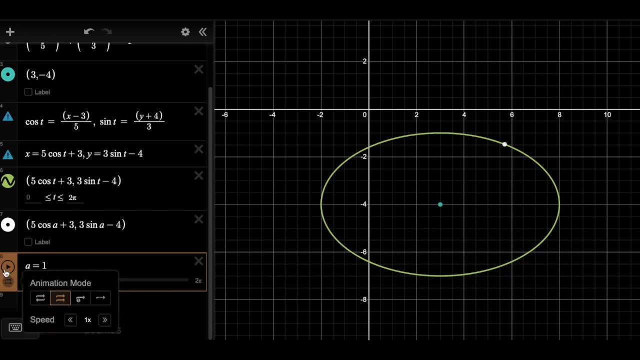 pi, We can actually watch its travel around this ellipse. I want it to start right at the beginning, So that's over there, at the point 8, negative 4.. And we'll watch it travel all the way around From 0 to 2 pi. And so this is one way you can define an ellipse using parametric equations. 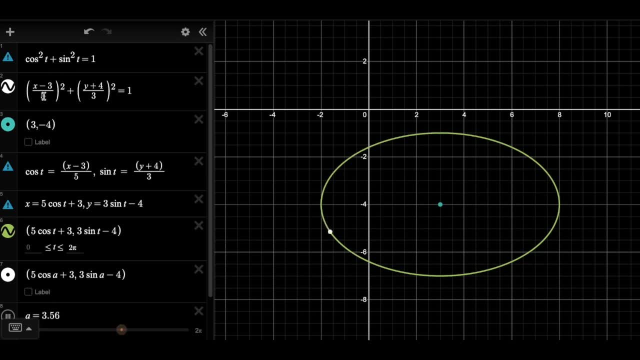 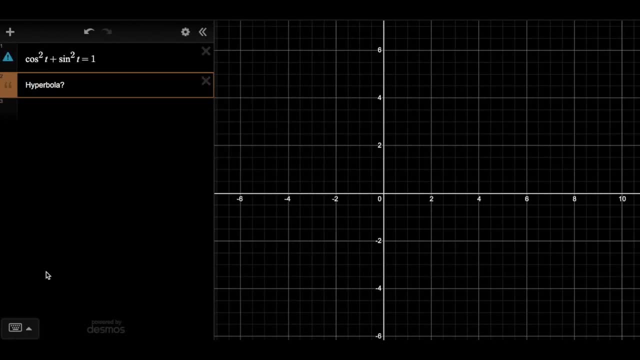 You make a direct comparison to cosine squared plus sine squared, solve for your x and y variables and you are good to go. So unfortunately, the hyperbola has a minus sign in it. So this cosine squared plus sine squared identity isn't really going to help us. We do remember that if we divide this identity, 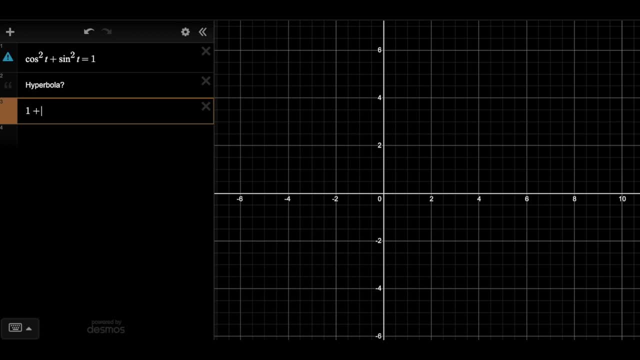 by cosine squared, we get 1 plus tangent squared equals secant squared. And another way to think about this identity is it's equal to secant squared minus tangent squared, which is equal to 1.. This has more of the flavor of our hyperbola. We have something squared minus something else. 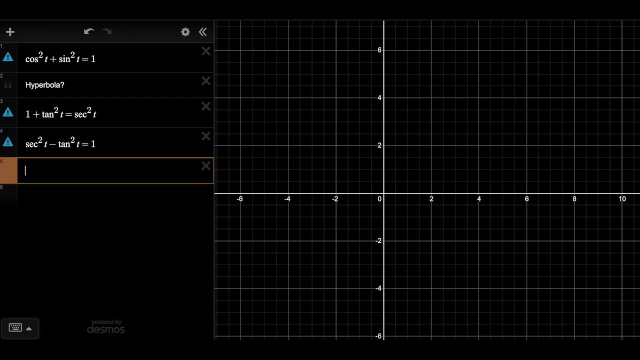 squared set equal to 1.. So if we directly compare this version of the equation to say, x over 3 squared minus y over 2 squared equals to 1, which, as we see, is a hyperbola, we can then make the substitutions, like we've been doing for the other conic sections. 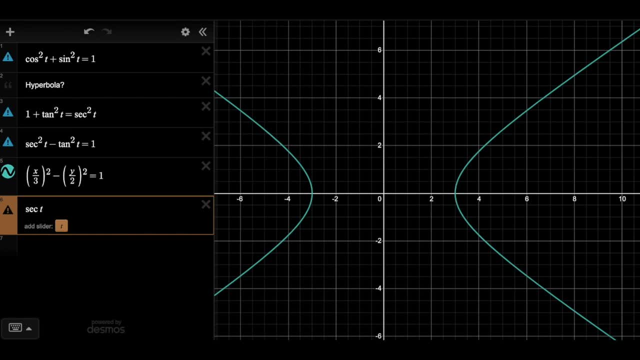 In this case, secant- is always going to be the positive quantity. So, in this case, being x over 3, which means that x is equal to 3, secant t- In this case tangent- will always be the negative quantity in the hyperbola, y over 2, which means that y equals. 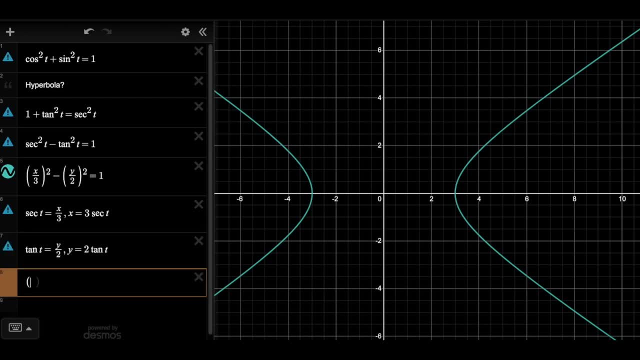 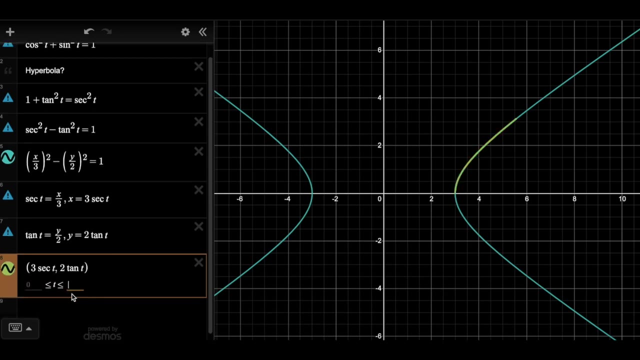 2 tangent t. So we can go and we can graph our parametric representation now that we have it. If I just asked you for it, you can just say x equals 3 secant t or y equals 2 tangent t. But I do just want to show you the graphs are equivalent. Again, you have to go from 0 to 2 pi. 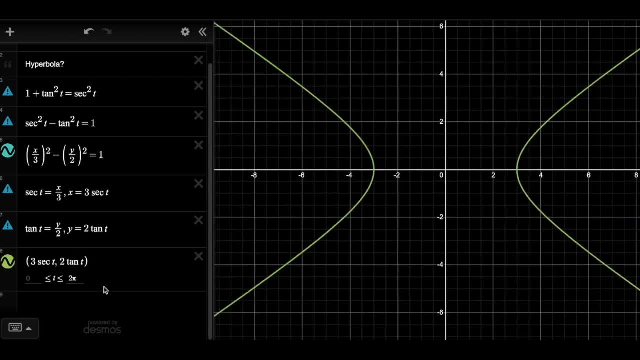 to get the entire graph. So be careful. This one, it matters a little bit more versus the sine and cosine. You have to make sure you make the positive quantity secant and the negative quantity tangent. or this: secant squared minus tangent squared equals 1. identity will not hold true. I ignored, probably the most. 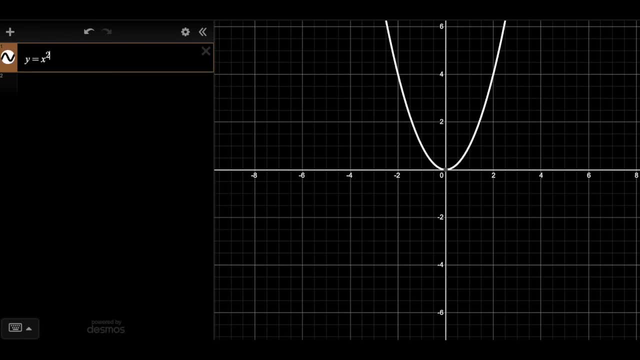 basic conic section, your very famous parabola. And so you might be thinking to yourself: well, there's definitely no x squared cosine, squared sine with one squared and one not squared identity. And that's because parabolas parametric. 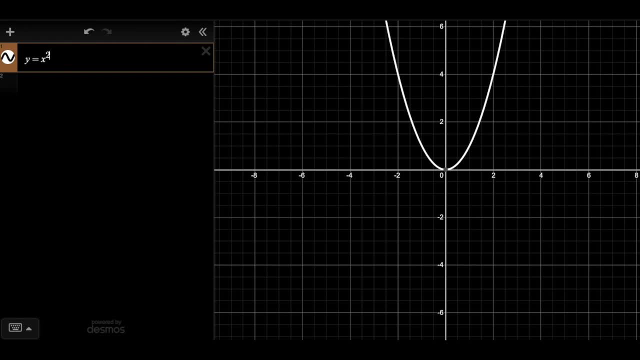 representations don't involve trig functions. They're the only ones In this case. if you just say, let t x equal to t, well, if y is equal to x squared, then y is equal to t squared in this case. So we have the representation t, t squared, And so if you go, 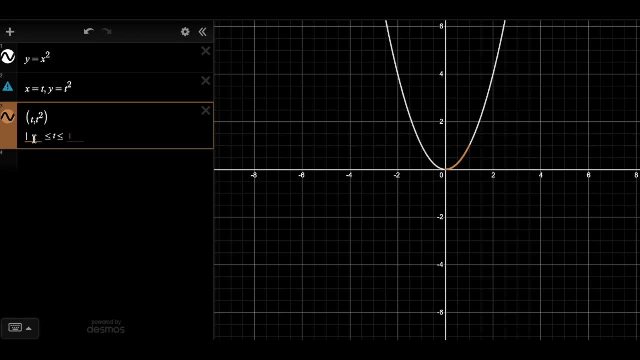 in this case, because it's not trigonometric, you actually have to find all possible values of t to graph the entire parabola. So you can make much fancier parabolas. You can say 4 x squared minus 1.. If you have something like that, again your independent variable. 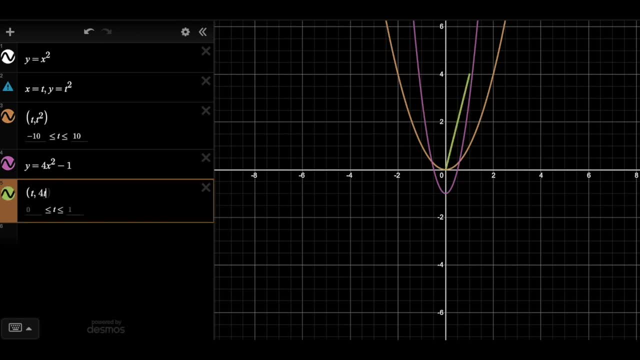 in this case, which is x. your y is just the original equation written terms of t. So parabolas are just a little bit more boring and that's why we don't spend as much time on their parametric representation. I always say it's just as important to know the 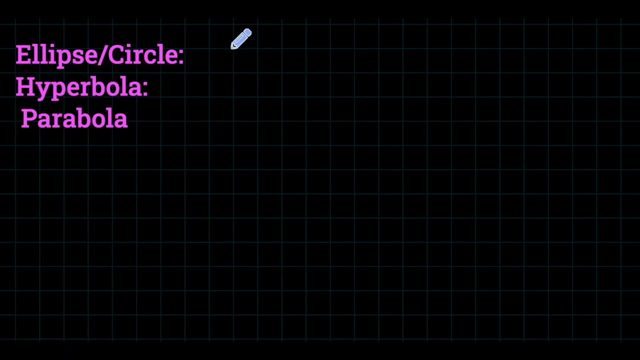 formula as to know where the formula comes from. So again, the ellipse and the circle are all based off this identity that cosine squared t plus sine squared t is always equal to one. That's our favorite Pythagorean identity. It does not matter so much in the ellipse circle situation which 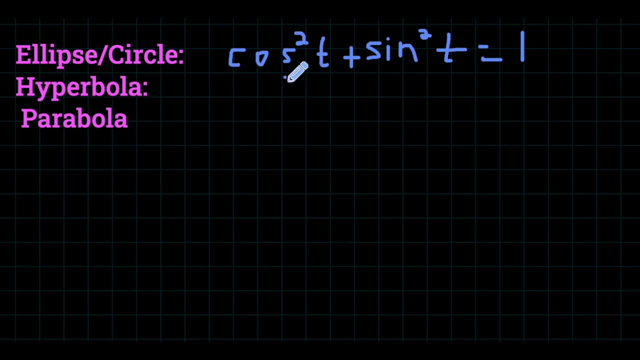 variable you define to be cosine or sine. In some cases it might make more sense to do x or y or y or x. While it won't affect the overall shape, if you define it on its entire domain, it will change starting point and direction. The hyperbola was based on a related Pythagorean. 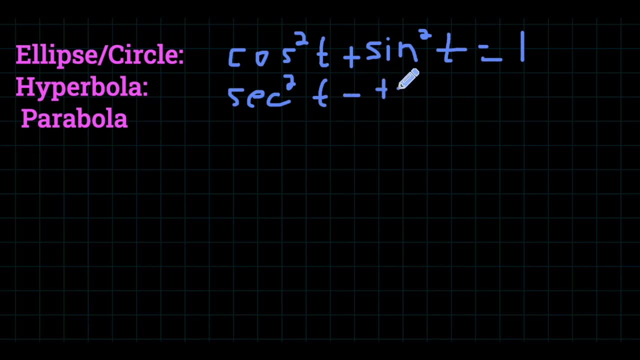 identity. secant squared minus tangent squared is equal to one. In this case, it does make a big difference as to which one you're defining to be secant versus tangent. Secant's always the one that's positive in the hyperbola equation, and tangent is always the one you're subtracting. 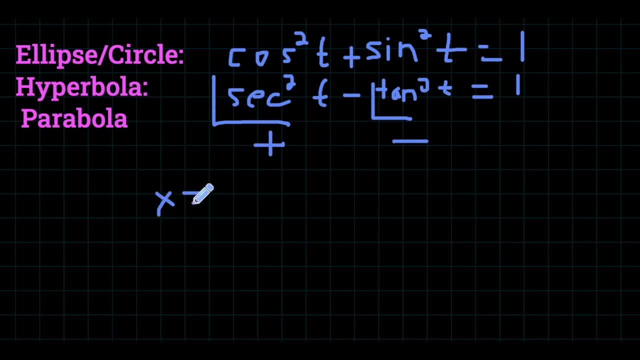 Parabolas. unfortunately they're just not as exciting to define. So say you had x equals y squared plus four. You would say: let x equals y squared plus four. You would say: let x equals y squared plus four. You would say: let. 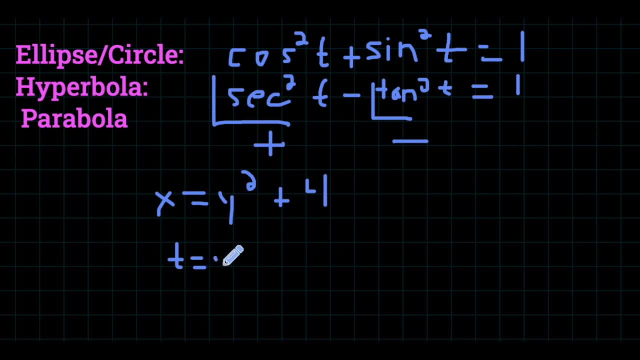 t be equal to y, and thus x is equal to t squared plus four. So not the most entertaining, not the most trig-oriented, but again it will complete our set of parametric equations of conic sections. So hopefully this clarified some things from the assignment and let me know if you have any. 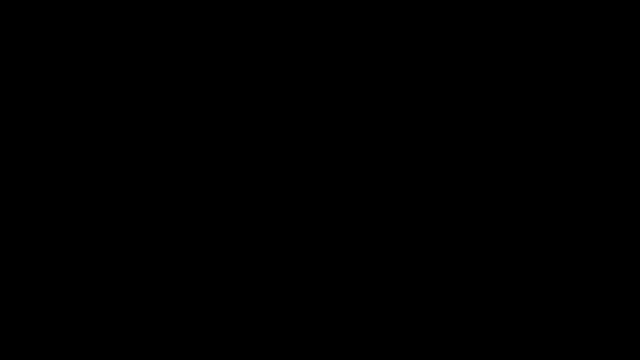 Thank you so much for watching and I'll see you in the next video.